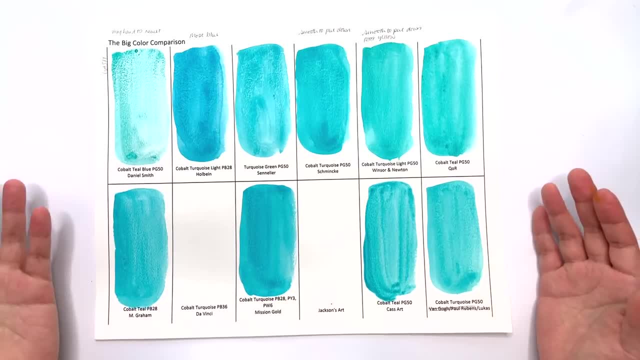 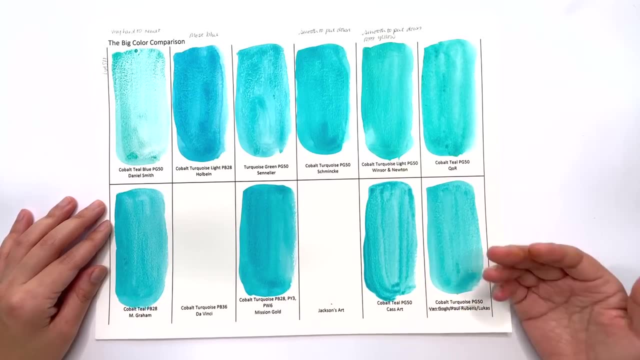 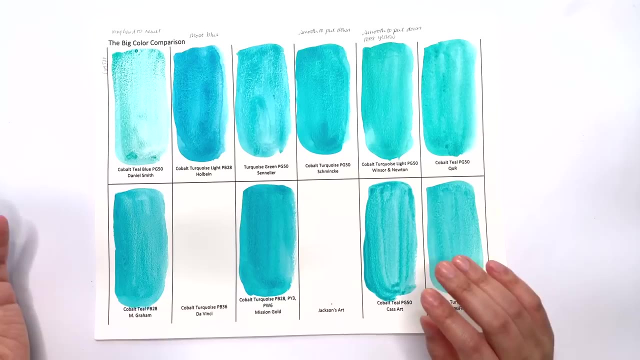 because, as beginners, we tend to just go by color name before we learn the pigments, and I want to show you how varied and how you can't quite rely on color names alone. However, in this episode I have to make an exception, because a lot of brands 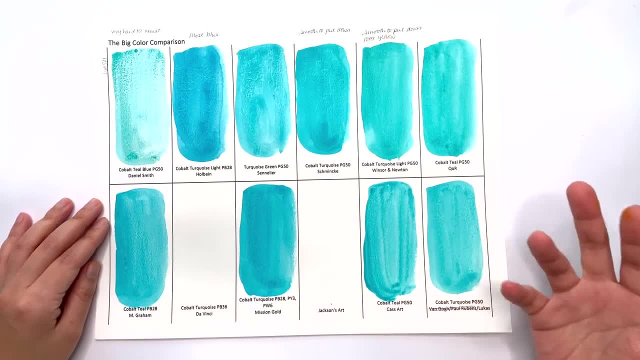 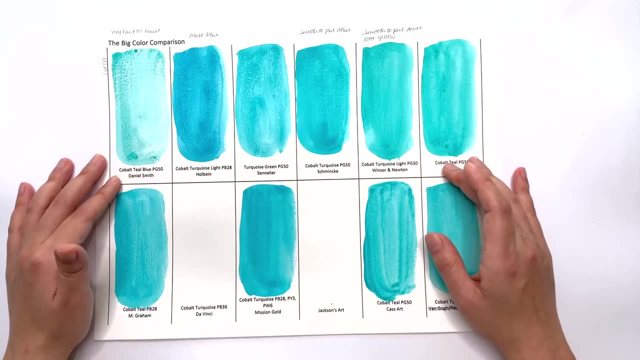 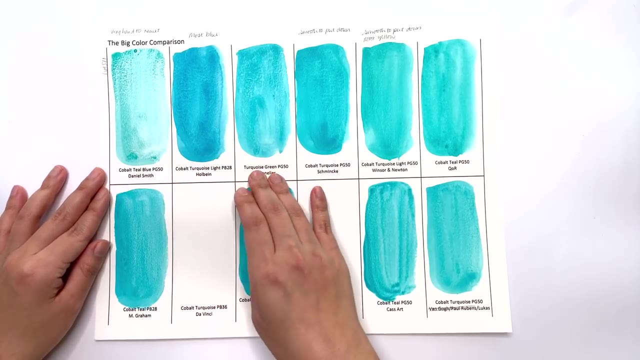 have a lot of different names for this tealy color that we're looking for. Some call it cobalt teal, something like cobalt teal blue or cobalt teal, and others call it cobalt turquoise- like cobalt turquoise, cobalt turquoise, light turquoise, green. So it was necessary to just go by the kind of 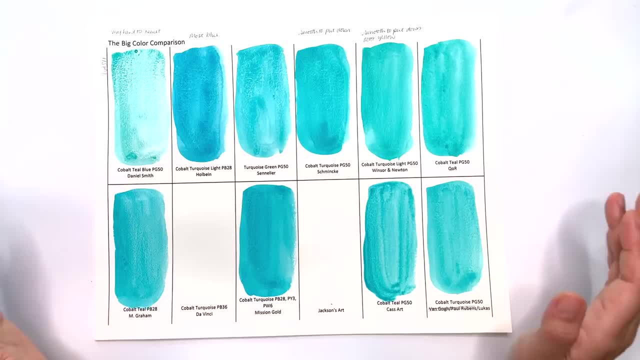 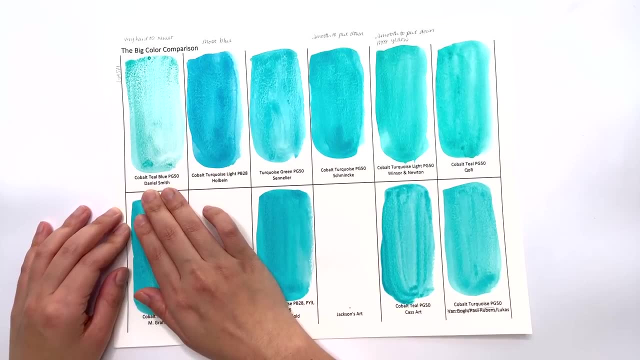 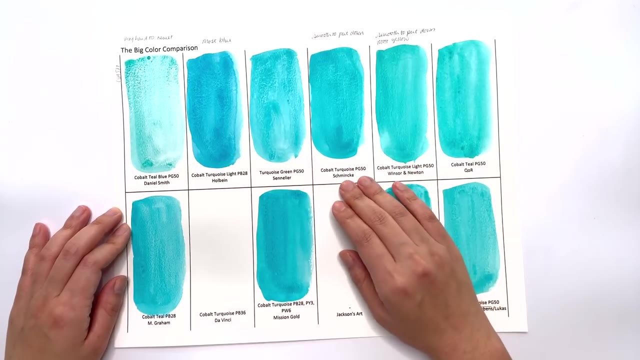 shade of color that we're all looking for when we think of the cobalt teal color. So the colors we have for this episode is: cobalt teal blue by Daniel Smith. cobalt turquoise light by Holbein. turquoise green by Sennelier. cobalt turquoise by Schmincke. cobalt turquoise light by Windsor. 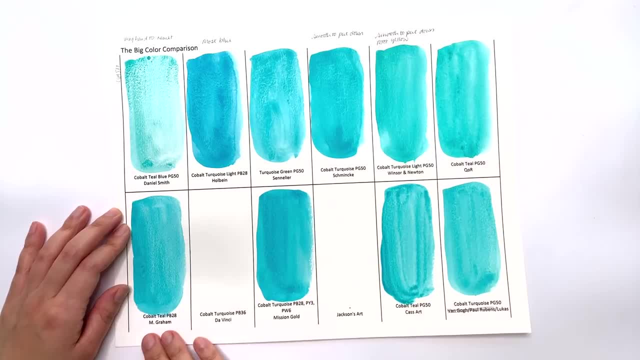 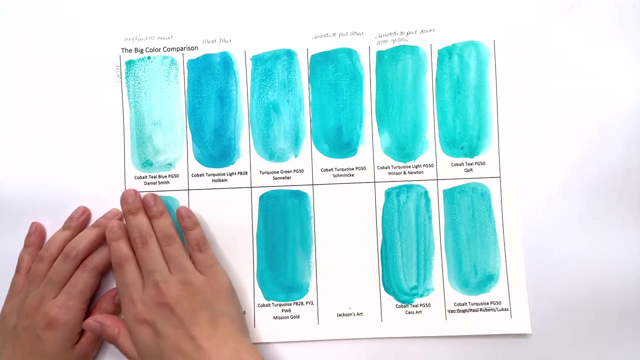 Newton, cobalt teal by Kohl, cobalt teal by M Graham, cobalt turquoise by Mission Gold and Cass Arts cobalt teal, as well as the cobalt turquoise by Lucas. Most of the colors are PG50.. The Daniel Smith, Sennelier, Schmincke, Windsor, Newton, Kohl. 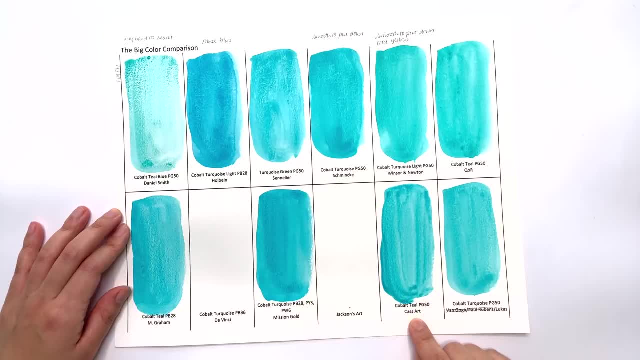 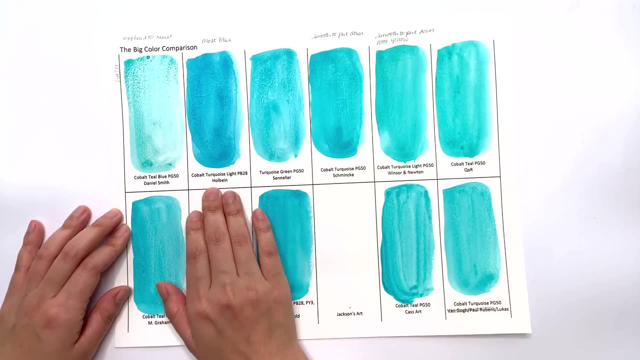 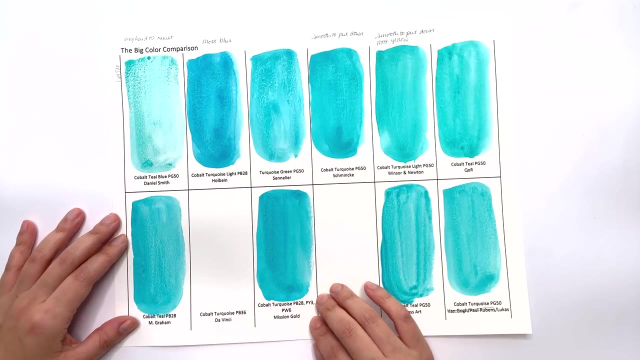 as well as the cobalt teal by Cass Arts and Lucas's one, are all made out of PG50.. The exceptions are Holbein and M Graham. both use PB28, and then, for some weird reason, Mission Gold felt it necessary to mix three pigments: the PB28, which is the same as Holbein, 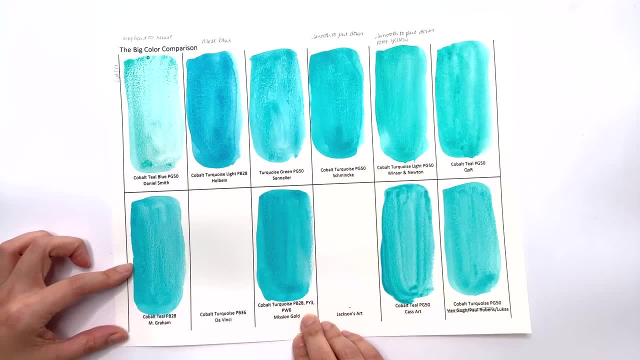 M Graham, as well as PY3, a yellow pigment, as well as PW6, that's white, and I have to say, for mixing three colors it hasn't really made that much of a difference in terms of hue. It's definitely different from this, but the Holbein one was different from M Graham anyway. so if you do, 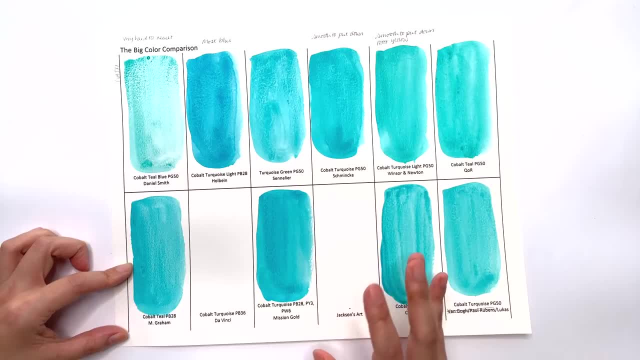 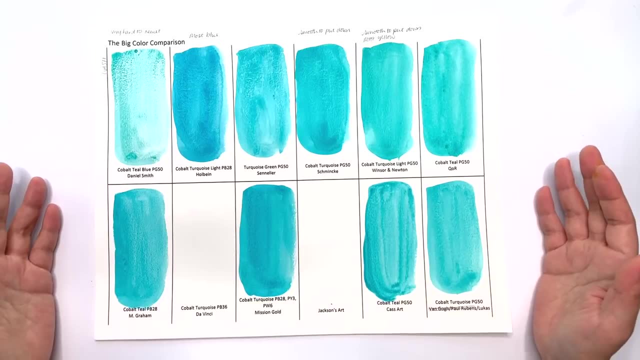 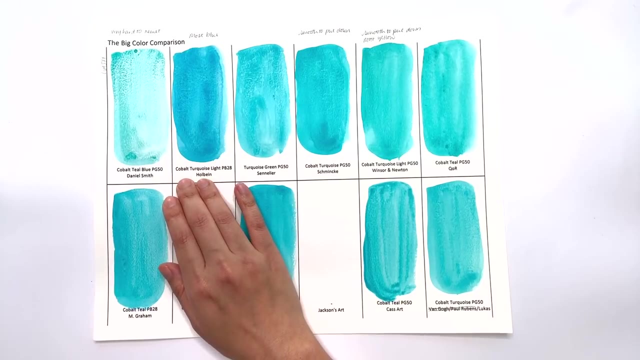 get a little bit twitchy about multiple pigments in an unnecessary way, then I would avoid the Mission Golds. For each brand I just picked a color that was closest to the color we think of when it comes to cobalt teal. However, Holbein's one is the most blue out of all the teal colors. This is as tealy. 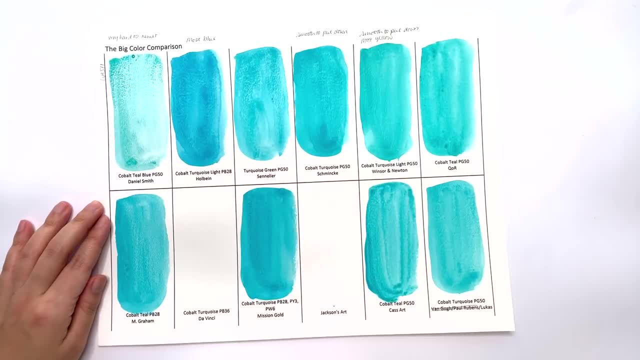 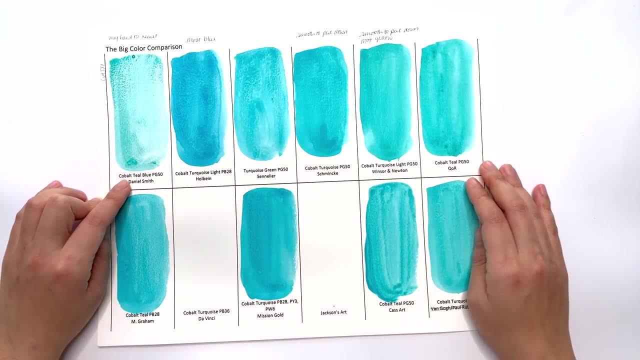 as Holbein gets. I would say the most green one is the Daniel Smith one and it's also noticeably more granulating than all the other colors. It's then followed by over here the M Graham one, the Winsor & Newton and the Kohl one. They're very nice, slightly green, tealy color On the. 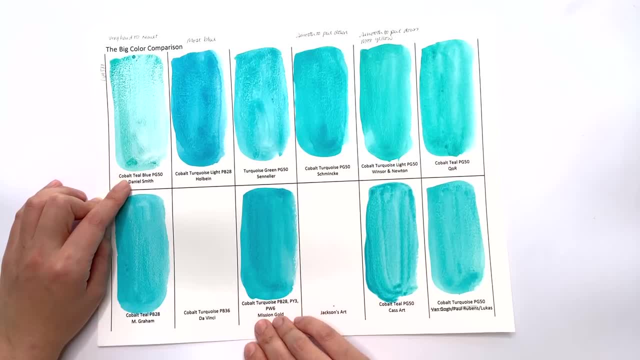 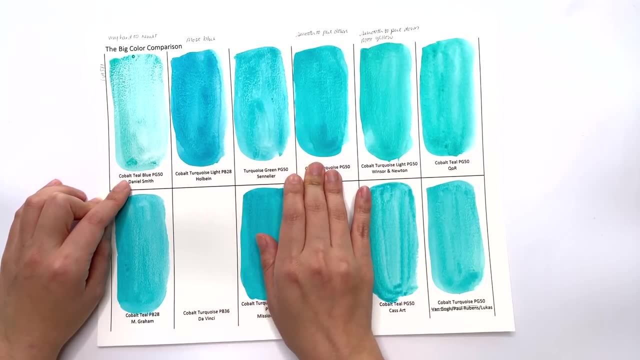 bluer side we have Mission Golds, which is a step more green than the Holbein, but it's still on the bluer side, as well as Snellier and Schmincke, and in the middle we have M Graham and Cass Art and 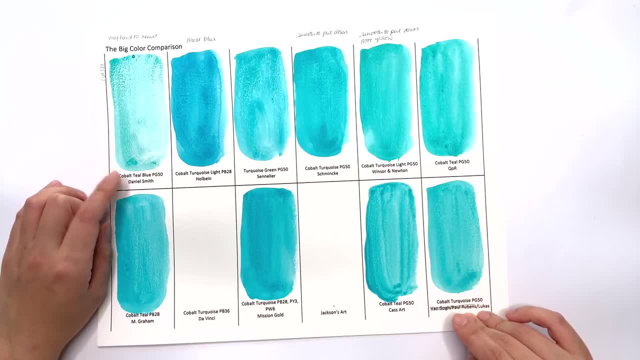 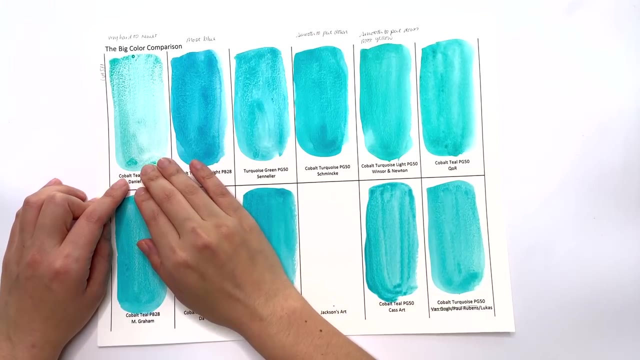 the Lucas one. One thing I do have to mention is that the Daniel Smith one was incredibly hard to re-wet to all the other colors. I just had to sit there and scrub away at the color to get any kind of color. it doesn't have a high tinted strength, it's more of the 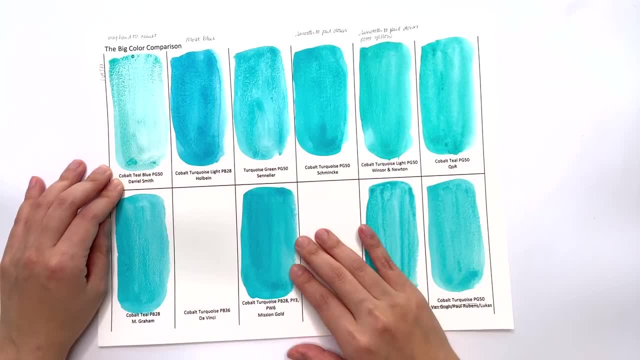 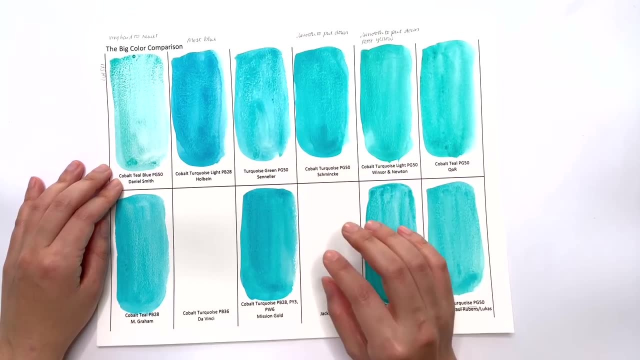 particles in it are colored rather than an overall color. the Schmincke as well went down very smooth, as it has been for the whole series. I'm very impressed at how Schmincke colors are such a joy to put down on paper so far in this series. 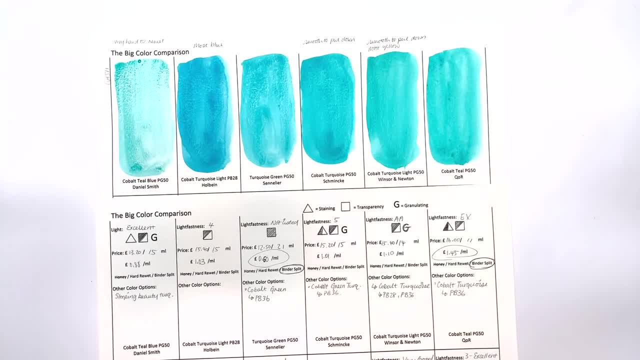 let's look at the prices next and, not surprisingly, cause one is the most expensive by being 1 pound 45 pence per milliliter. the prices are UK prices. I've taken them from Jackson's so that we can compare the UK prices, if you're. 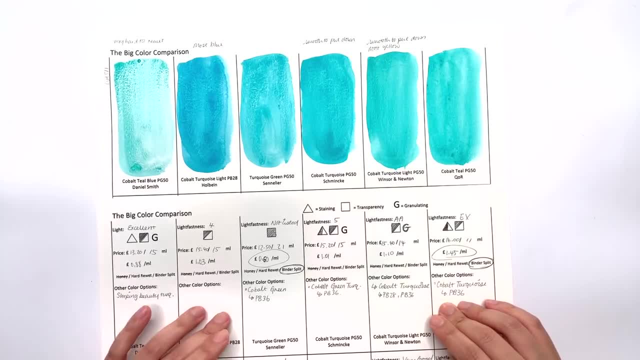 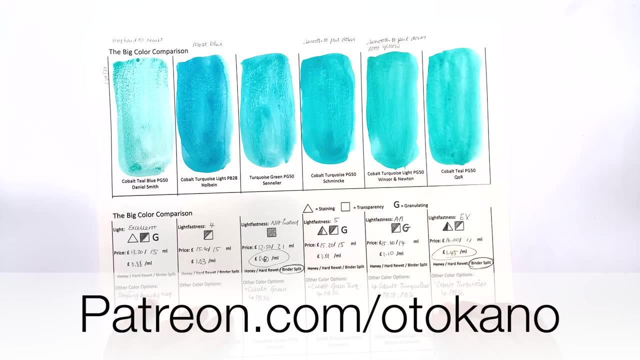 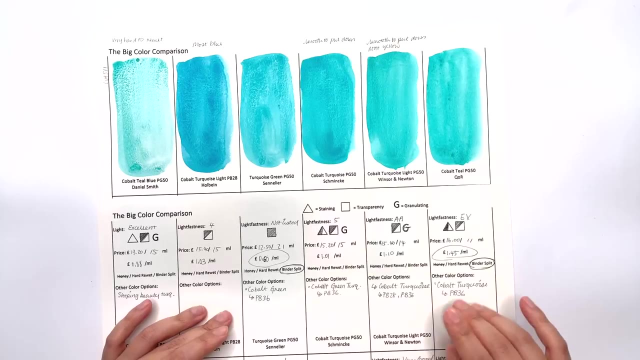 interested in the US prices. a very helpful patron has been listing the US prices for us over on my patreon, which is patreoncom forward slash otakano. so thank you, christina Todd, for all the hard work in doing the research for us. the cheapest one is: 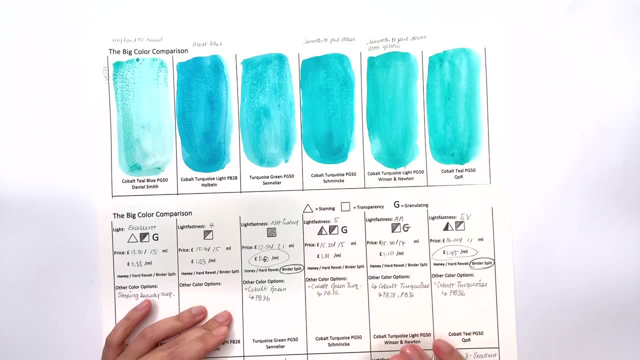 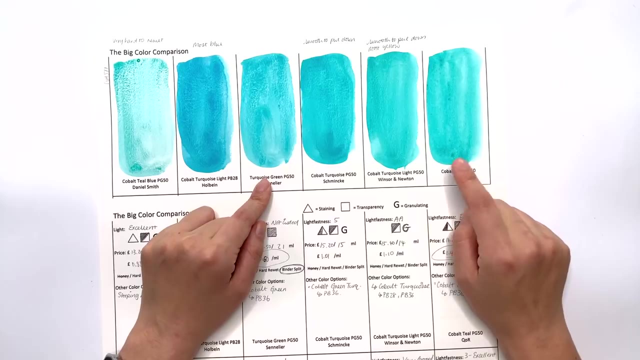 normally the Jackson's, but because the Jackson doesn't have a TD turquoise color, it is the Sennelier's- is the cheapest by being 60 pence per milliliter. that's less than half price of the core one. so this and these, this is more than. twice the price of this color, although I do have to say I do love the hue of the coarse cobalt teal. however, Winsor & Newton's one is very similar in hue and that's a lot cheaper at one pound 10 per milliliter. so if you do want to save a, 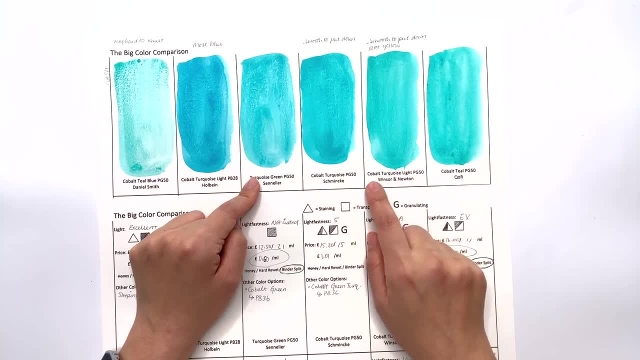 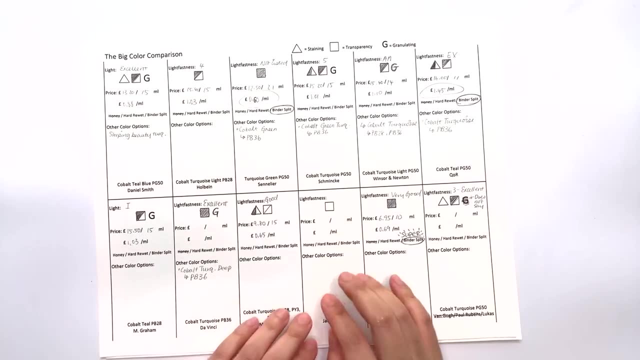 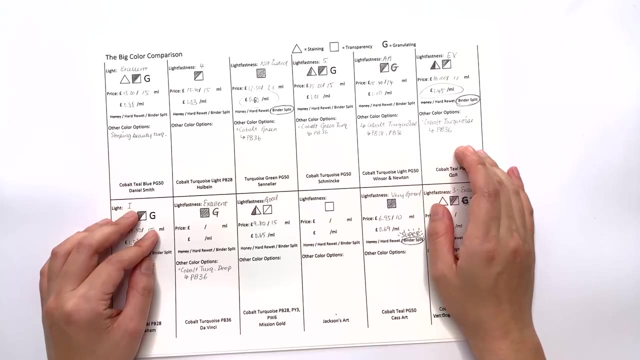 little bit of money. then you could consider Winsor & Newton one. one thing I have to mention while I'm using this info sheet is how many of the colors split from their binder. the Sennelier's one, and even coarse one- surprisingly for the price had some binder that split from the 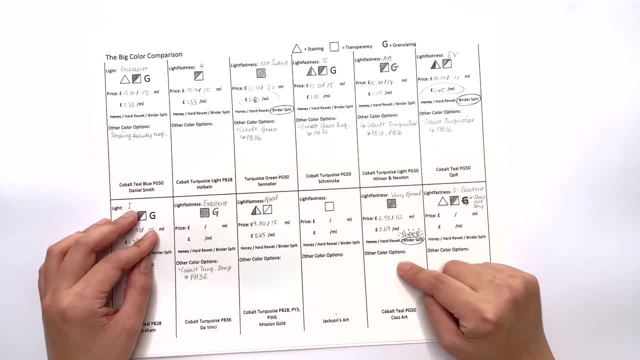 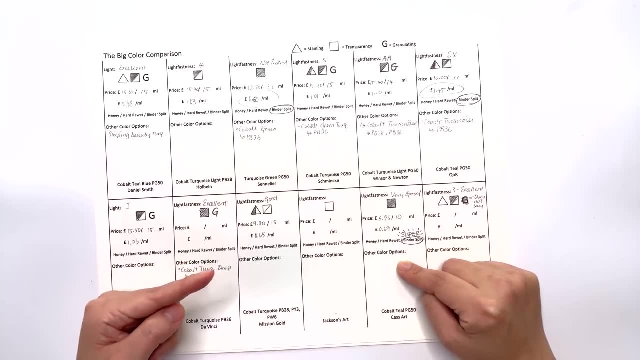 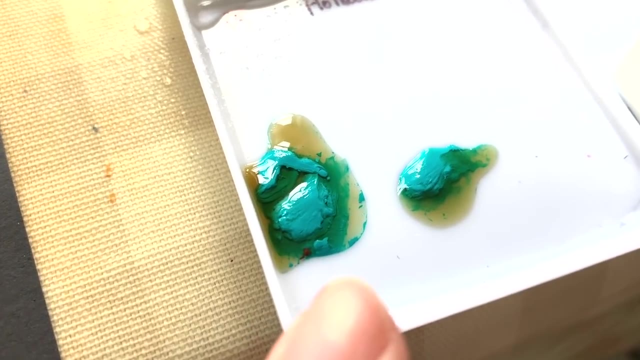 pigment. however, the worst culprit was Cassart's one, and I will show you a little video that shows how bad the binder split was when I poured paint out on the palette. just wanted to show you how much binder came out of Cass's paint. I think there's actually more binder than pigment or paint that came out of my two. 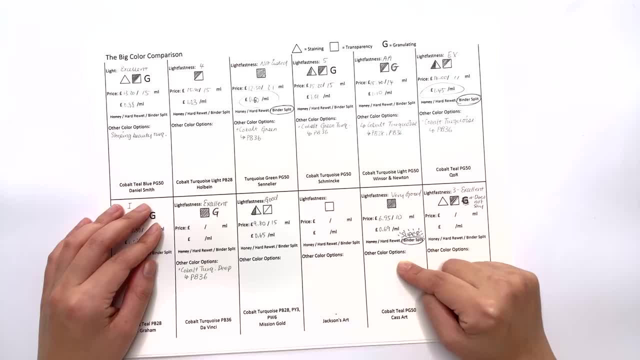 from Cass. as you can see, the binder just was horrendously split from the pigments and I kept pouring out more paint to see if it would get better and it just kept pouring out more split binders. so I have to say I would not recommend Cassart's cobalt teal whatsoever. of course a binder split can. 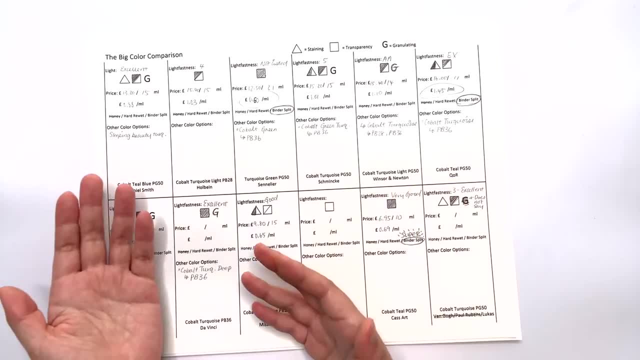 be caused from many different reasons. it could be different reasons. it could be because of the colour of the paint. it could be different reasons. it could be because of the colour of the paint. it could be that the paints have been sat there for a longer time than the other colours we. 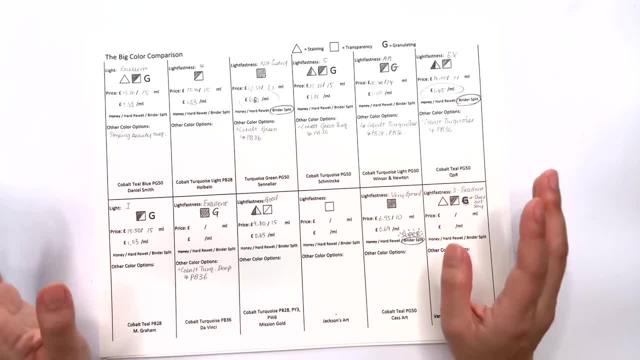 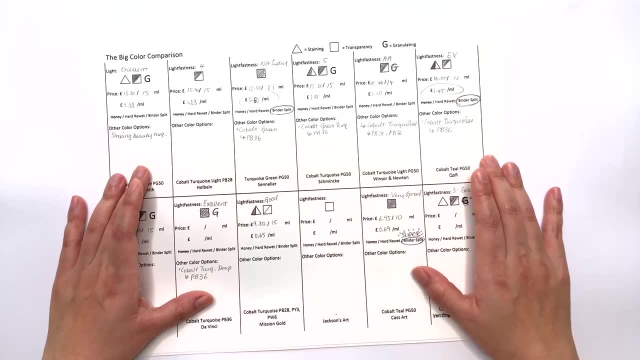 just don't know what really causes binder split, but with cobalt teals I do definitely notice more binder split across the colour than any other colour we've covered so far. it doesn't, of course, mean that the tube you're gonna buy it from- either the Sennelier core or Cassart's- is gonna be as badly. affected by the binder split, and it also doesn't mean that the other brands are sure to not have binder split. cobalt pigments are quite heavy pigments so they do tend to split from the binder a little bit easier than other pigments anyway. so just be aware that when you're buying. 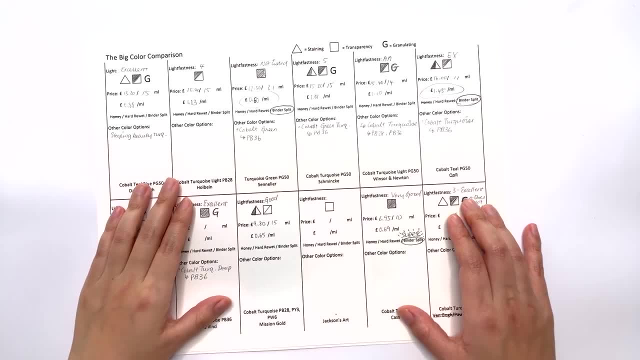 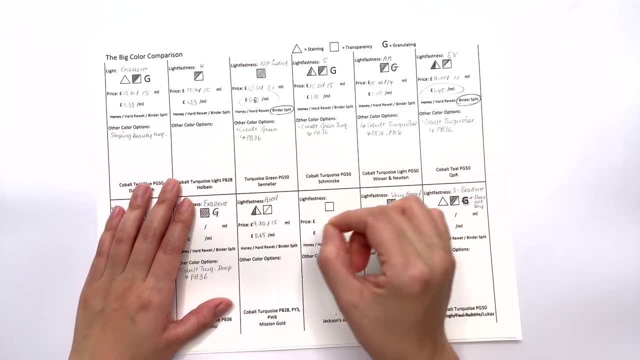 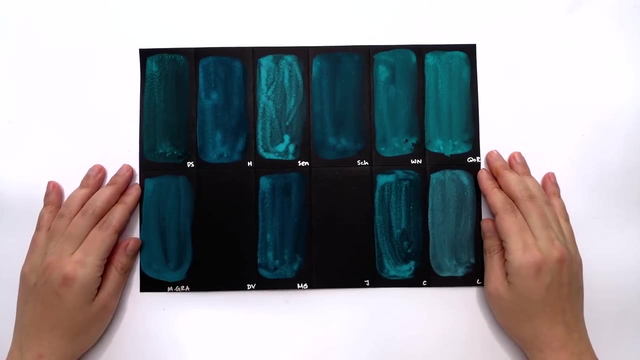 cobalt colours, you are going to experience more binder split. don't worry if you get some binder split, though, because all you have to do is get a toothpick and just mix it about again, and you should be okay. moving on to the transparency test- and cobalt colours tend to be very opaque, the most opaque. 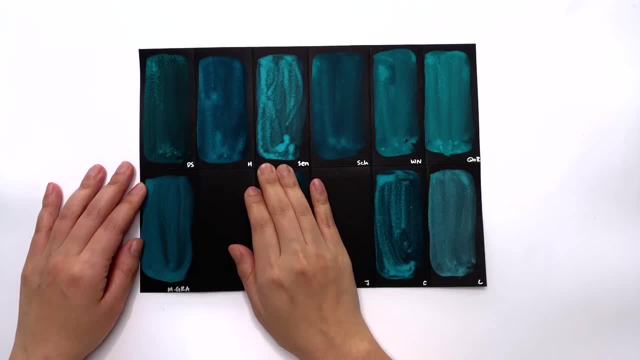 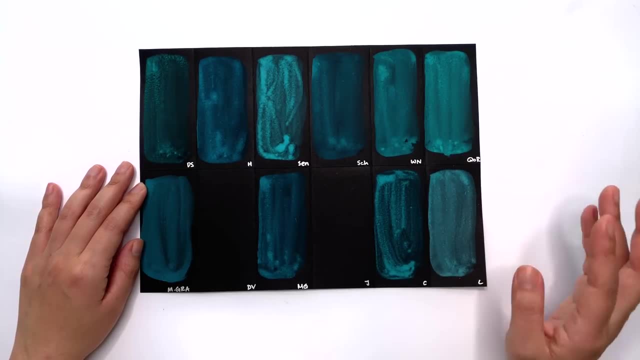 one out of the lot was the Sennelier's one. you can really see how much more opaque that colour is compared to the other colours. I would say that the three that are the second most opaque, and that's these three: the Winsor & Newton one, the core one and the Lucas one- Lucas one, it being a student quality colour. 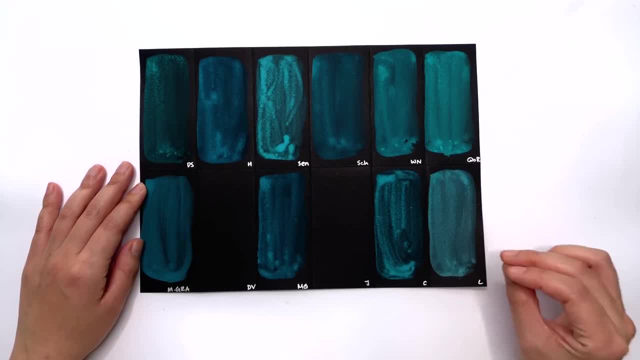 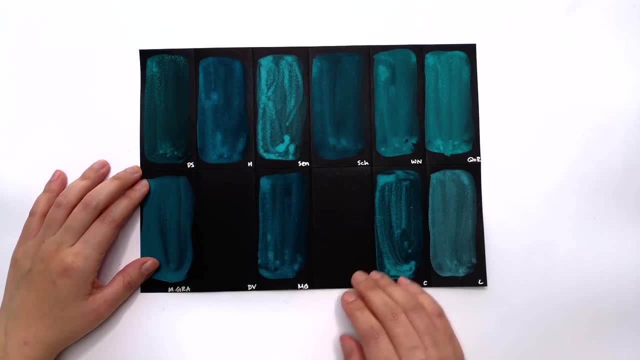 does seem to have whiteness to it, and that's probably a thing that you need to be very careful with. as you manifest with a filler. it's a different type of opacity to the other cobalt colours. it's more powdery over whiteness. the most transparent out of the cobalt colours without Daniel Smith. 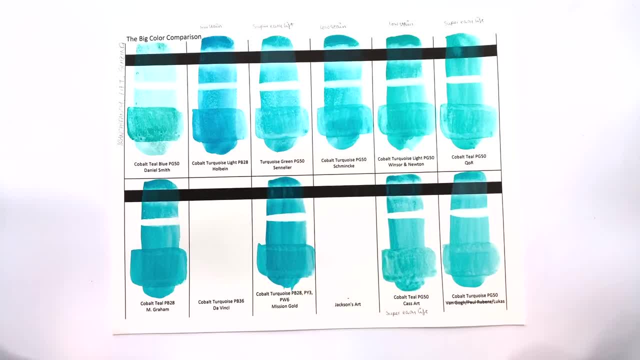 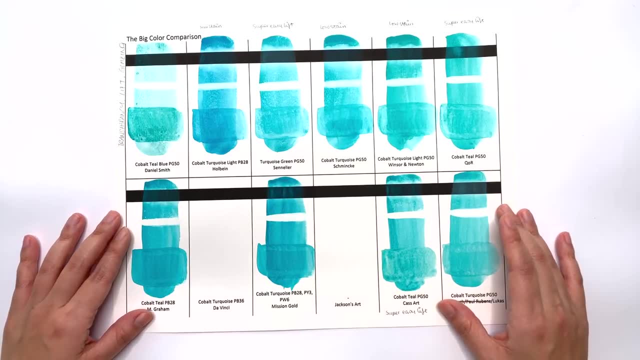 followed by Schmincke and then the Holbein and Graham and the Missions Gold are somewhere in the middle. now unto the lift, and with the cobalt tails it's very of. the colors will lift off very, very easily and very cleanly- Easiest colors. 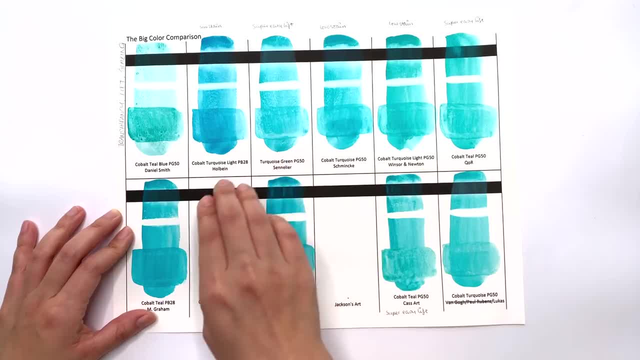 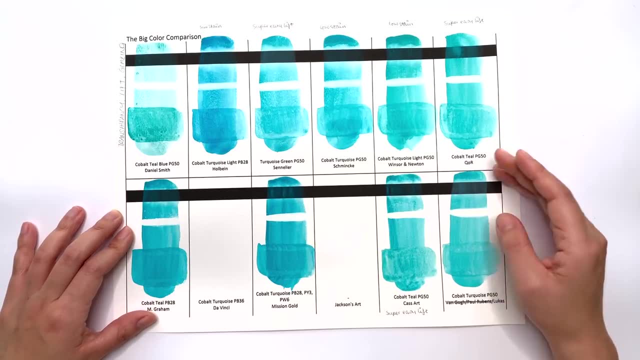 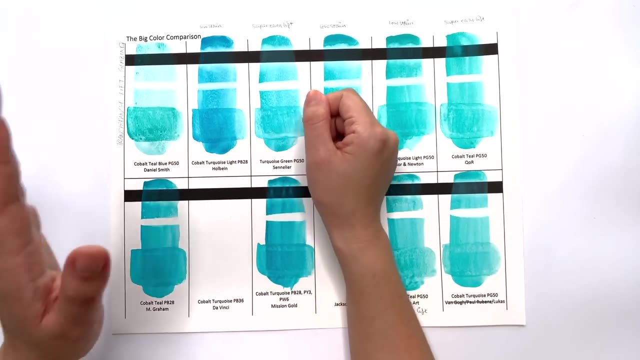 to lift were the Cobalt Teal by Cassarts, the Turquoise Green by Sennelier, as well as Cobalt Teal by Core. These came off almost back to white. When I do the lifting test, what I do is I swipe with a damp, clean brush three times and then 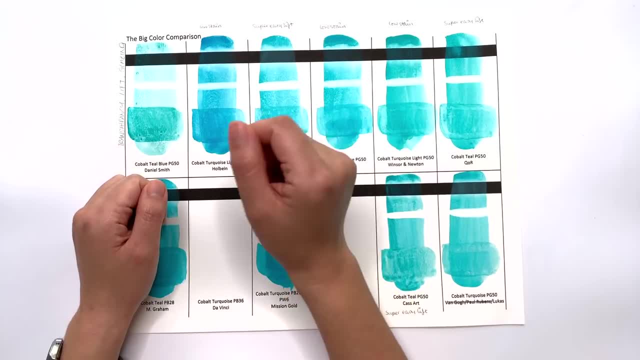 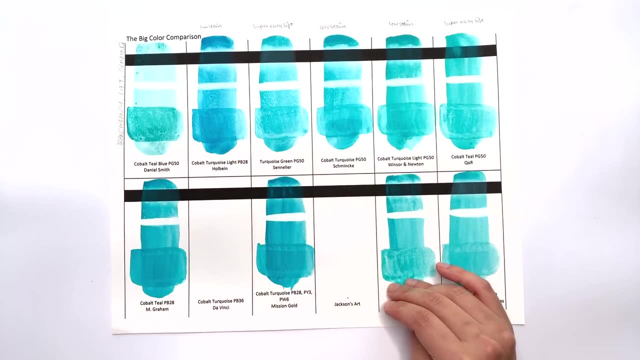 pat the area dry and then do that again. So I do it three times, three sets of three strokes, and with these three colors it was back to white after the second round, let alone the third round. So if you want a nice, easy lifting, 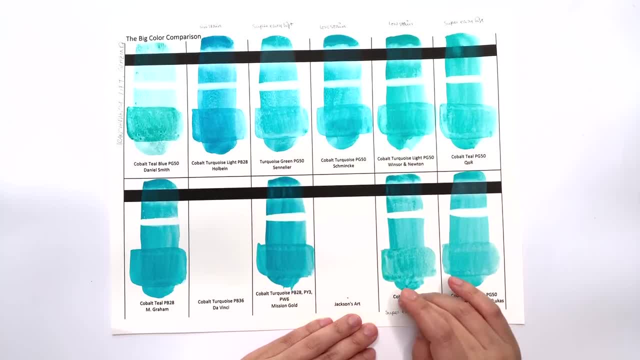 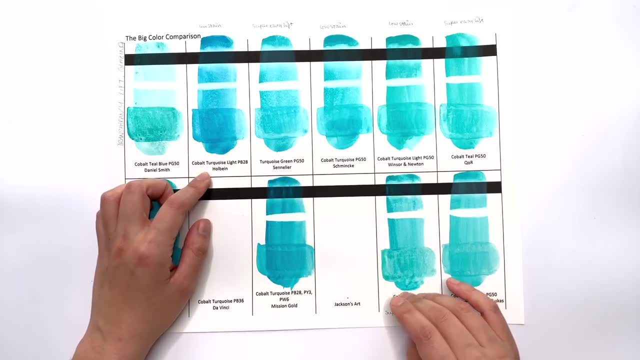 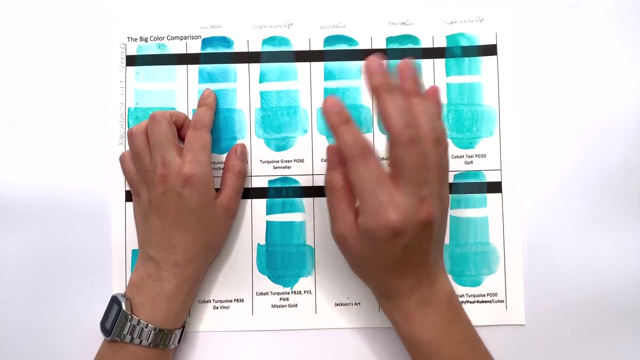 colors, I would go for Sennelier, Core or Cassarts. The most staining of the colors were the Cobalt Turquoise Light by Holbein and Schmincke's Cobalt Turquoise. They are still stained on the paper a little bit, even after three. 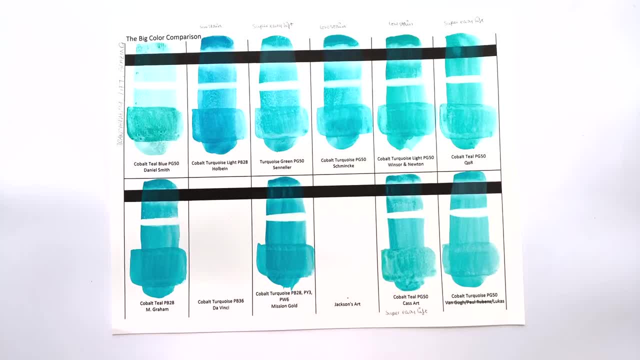 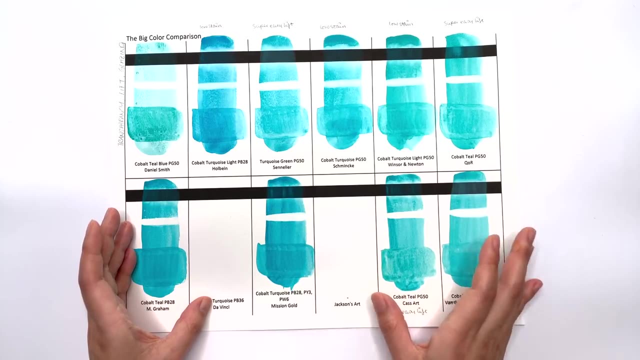 rounds. All the other colors lift it to a clean white by the third round of lifting In terms of glazing, because it's a very low staining color and it's opaque, it is harder to do glazing with and you can really see that in say like this: 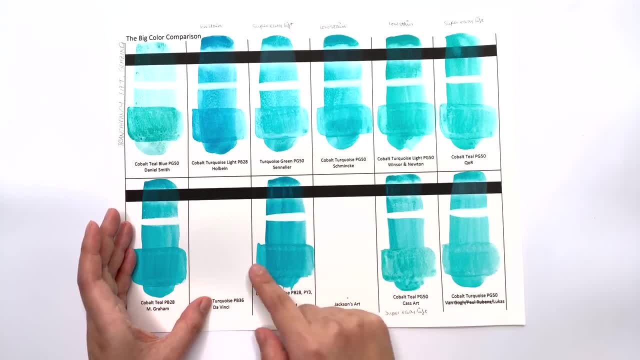 What I do is I go around, draw a box and then fill in the space that box in and you can really see where, when I go over it once and then go over that line again, the pigments in the bottom layer have really lifted, leaving this lighter edge and a darker box. 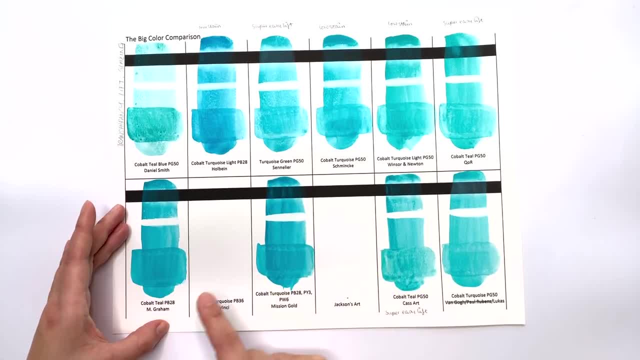 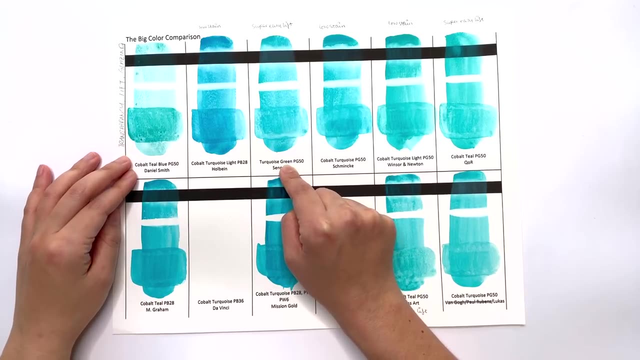 and you notice that a lot in the MGrams: one, Mission Gold's one, Lucas's one, Winsor & Newton's one and Quar's one and a little bit on the Sennelier's one. so if you do want to do layers with Cobalt Teal, it's not the easiest, you're not going to have the easiest time, but 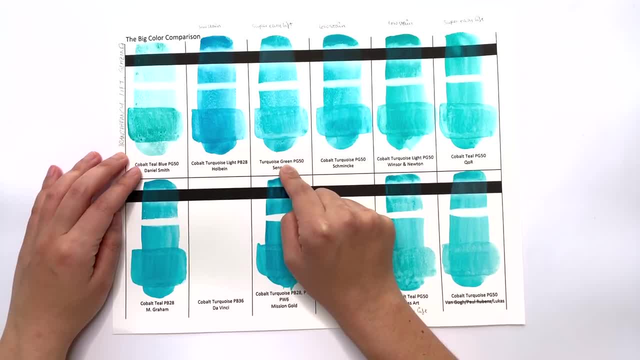 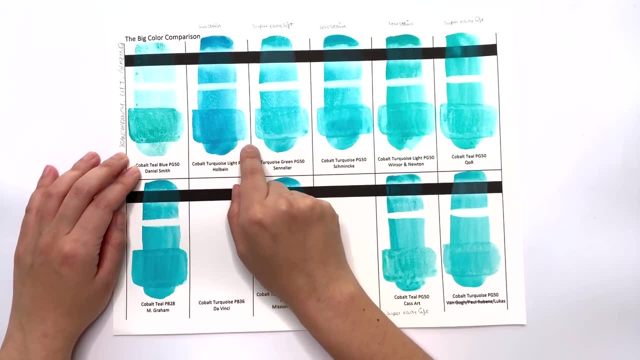 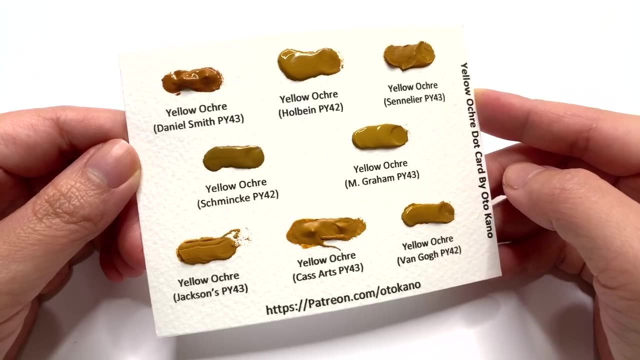 if you are going to do it, then I would stick to colours like Daniel Smith's one- it's pretty good- and Holbein's one, although Holbein's one is a little bit more blue than other colours and Daniel Smith's one, as we said, is incredibly hard to re-wet. This month's Patreon exclusive. 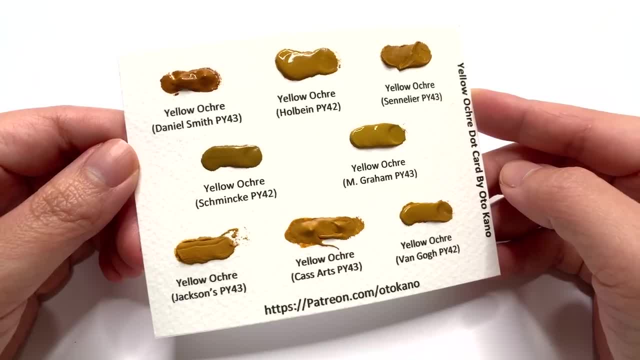 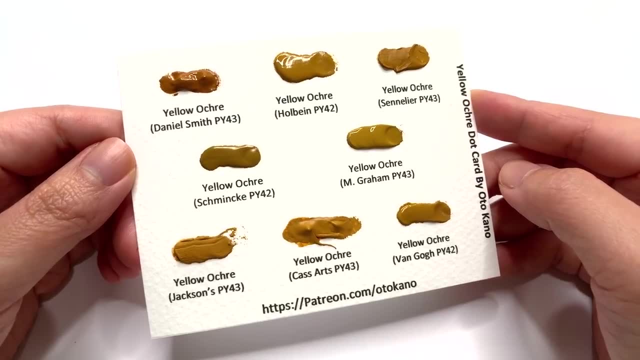 dot card is Yellow Ochres. Yellow Ochres for the third colour we covered in this series. and if you fancy carrying out your own comparisons, but if you don't want to commit to buying eight full tubes, then this is a really great economical way of trying out. 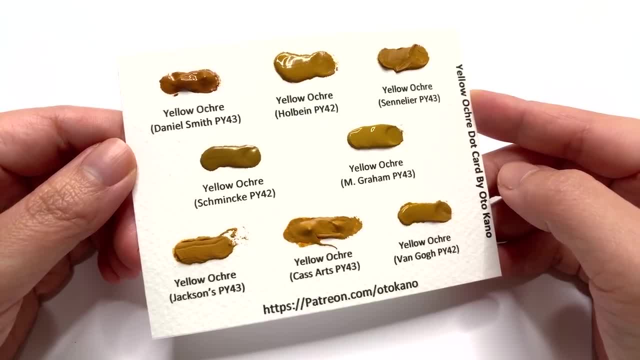 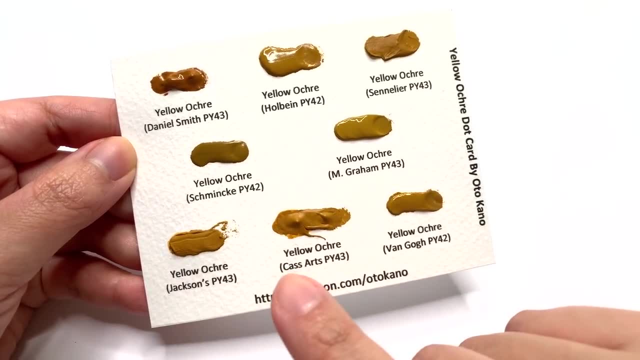 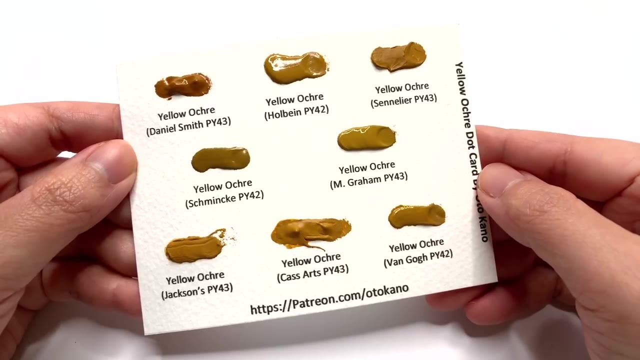 eight colours. You get seven artist quality colours: Daniel Smith's, Holbein, Sennelier, Schmincke, MGram Jackson's, Casas, and then you have one student grade of Van Gogh colour to carry. Yellow Ochre is your favourite. Yellow Ochre is a very fundamental colour in your palette. so 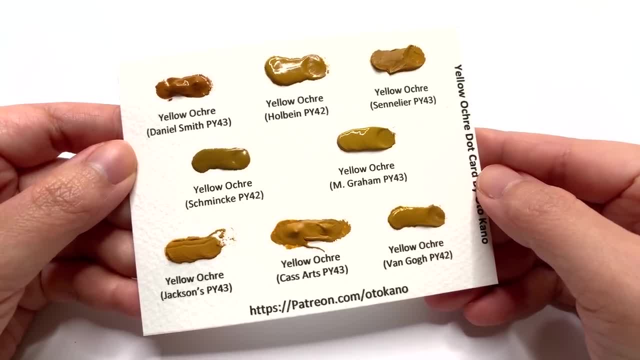 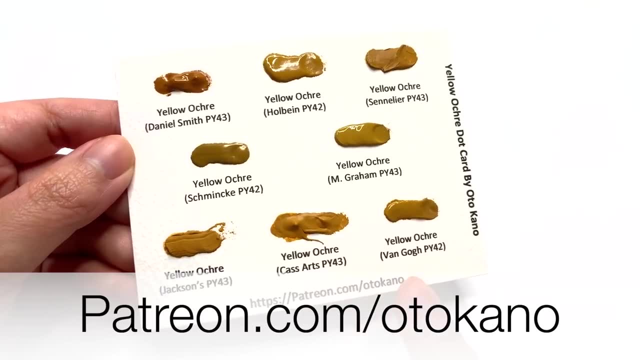 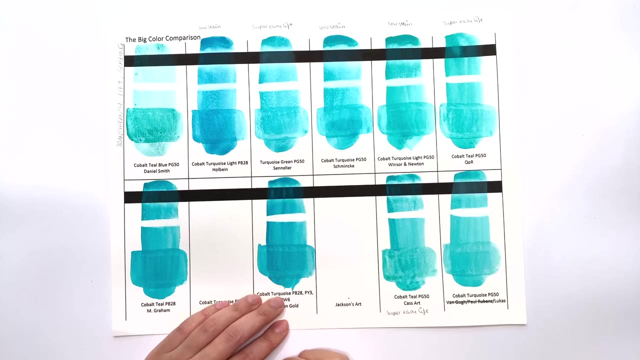 it's really good to be able to find the perfect Yellow Ochre for your palette. If you would like to receive this dot card, then do head on over to patreoncom forward slash autocarno, where you can sign up for the appropriate tiers to receive this dot card this month. So that's it for this.